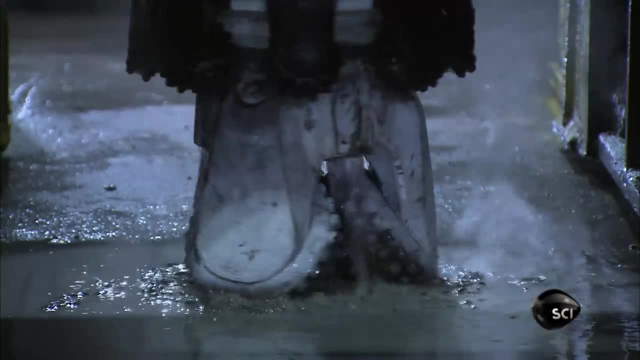 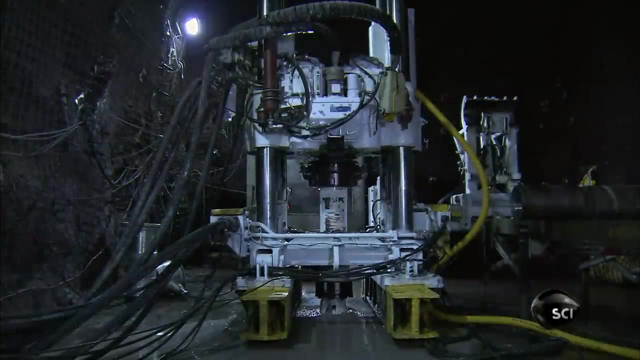 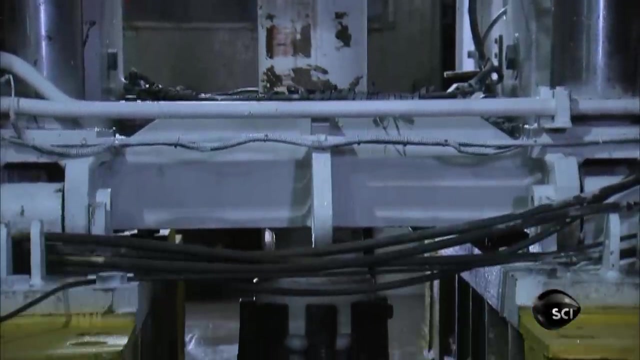 known as a pilot hole. The pilot hole maps out the drill route to ore and it creates an entry point for larger mining equipment. From a raised position, the bit bores vertically into the rock to drill the pilot hole and reach a specific level below the ore body. 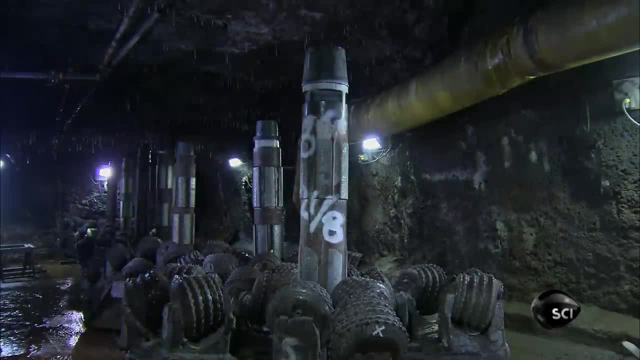 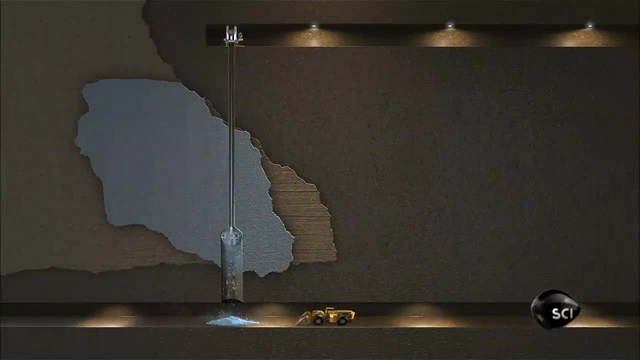 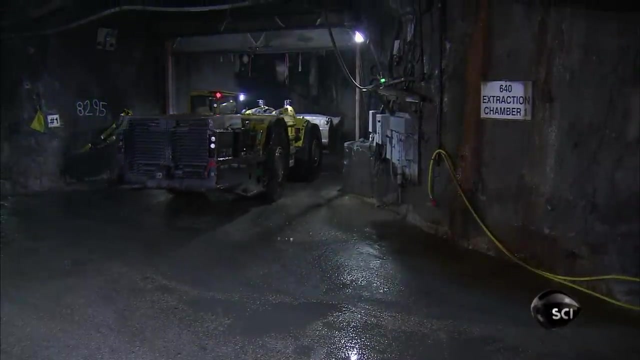 They're now ready for the reamer bit. The reamer has numerous button-encrusted wheeled tentacles, As this animation shows. the drill pulls the reamer up the pilot hole, widening it, and the broken ore falls into what's known as an extraction chamber. 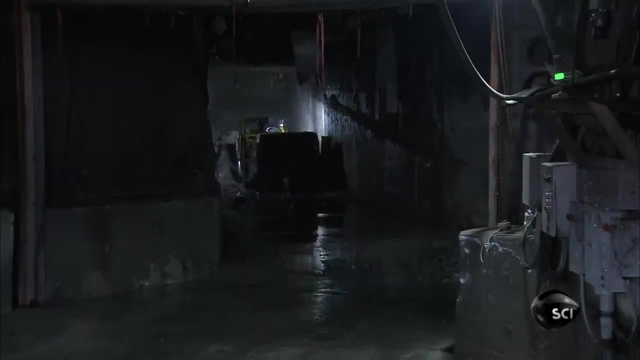 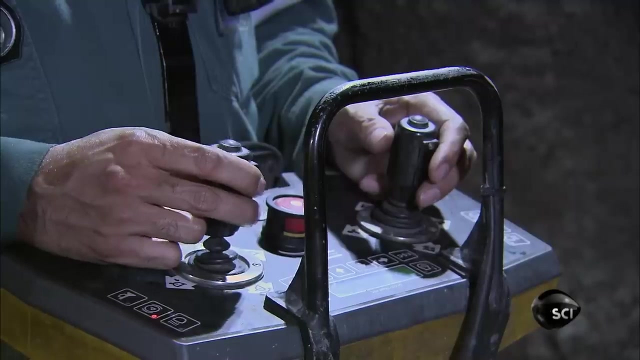 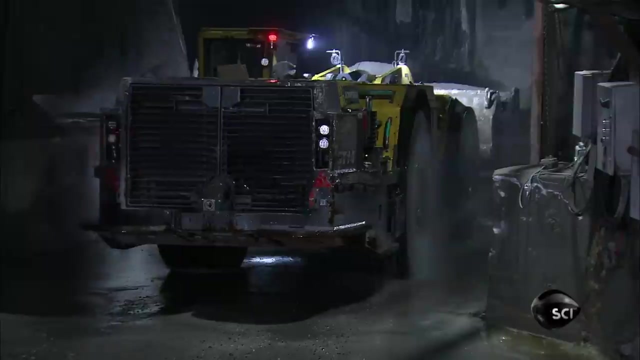 Here a tram operated by remote control scoops up the rock. This remote control system keeps miners a safe distance away from falling rock hazards. It also minimizes their exposure to the radioactive uranium in the ore. As another precaution, they continuously ventilate the mine. 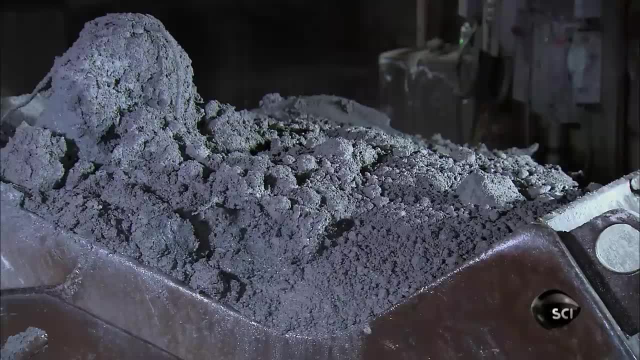 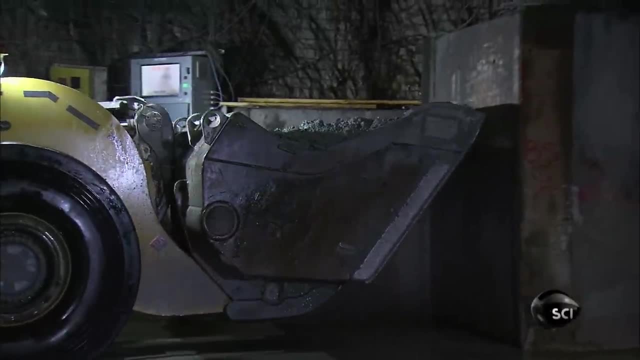 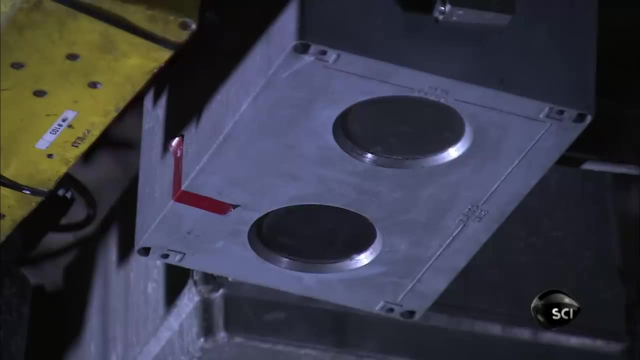 introducing fresh air every 20 minutes. Steered by the operator's joystick, the tram delivers the ore to a scanner. By measuring the amount of radioactivity in the ore, the scanner determines. the uranium content is about 15% In much of the ore. 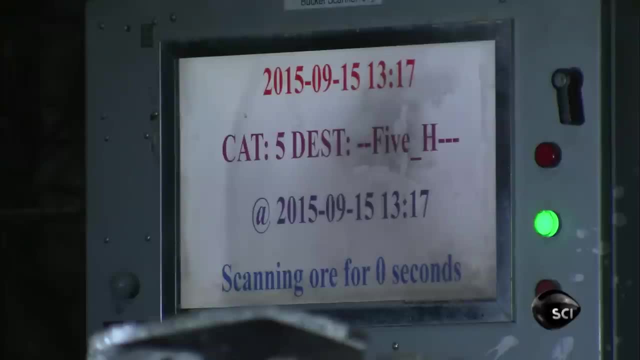 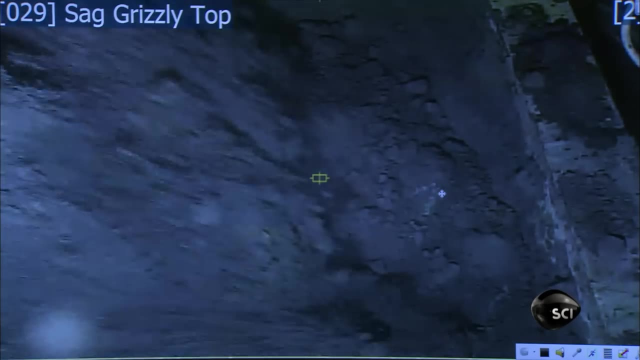 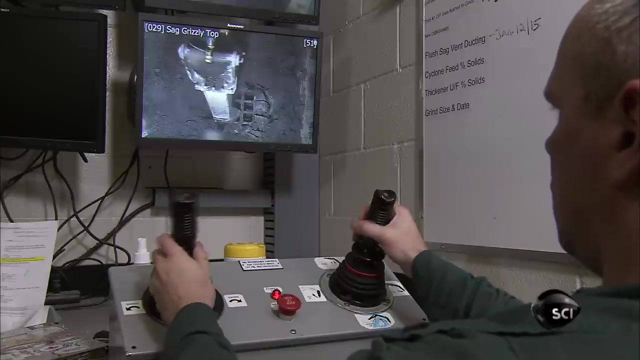 the uranium content is even greater, on average around 18%, and that's considered to be very high grade. The tram now empties the ore into a chute. Cameras follow the rock's journey to the next station, Then from a control room. 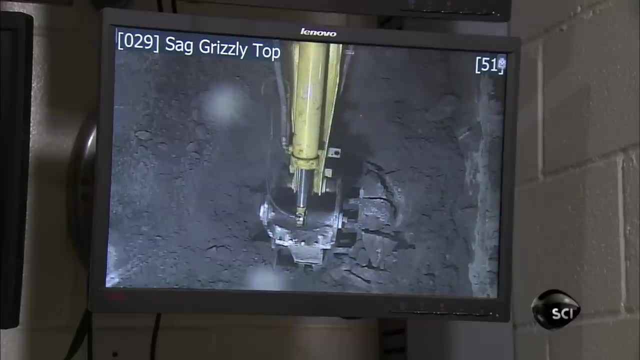 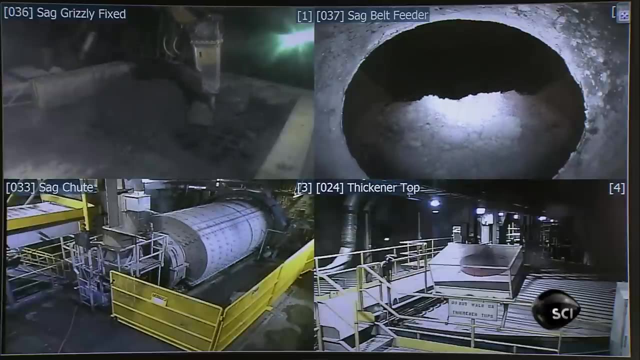 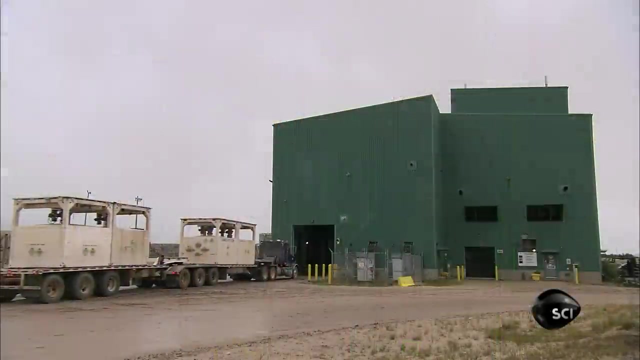 an operator manipulates a hydraulic hammer to smash the ore to bits. The broken ore then migrates to a mill that grinds it into a fine sand. They add water and it becomes slurry, which they then pump to the surface. Trucks transport the uranium ore slurry to a mill 80 kilometers away. 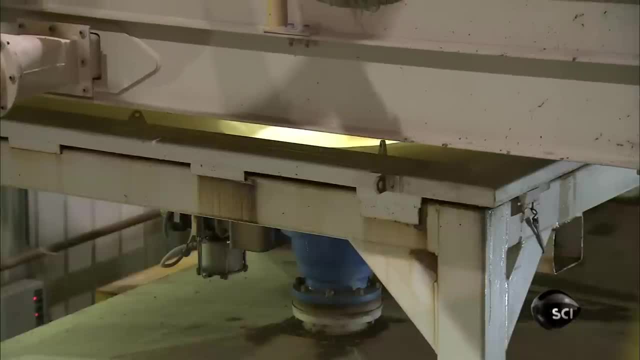 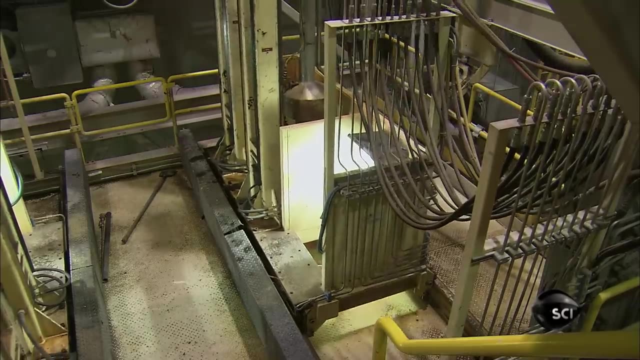 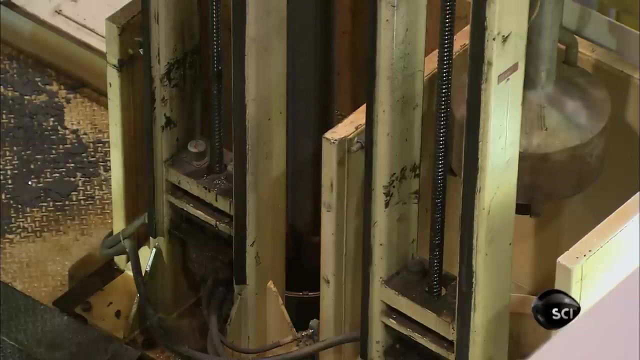 They pull into a special offloading facility. The support for a vacuum system aligns with the tote that encases the slurry tank. Once in position, a vacuum pipe drops into the tank and suctions up the slurry. Cameras provide a live feed of the unloading progress.